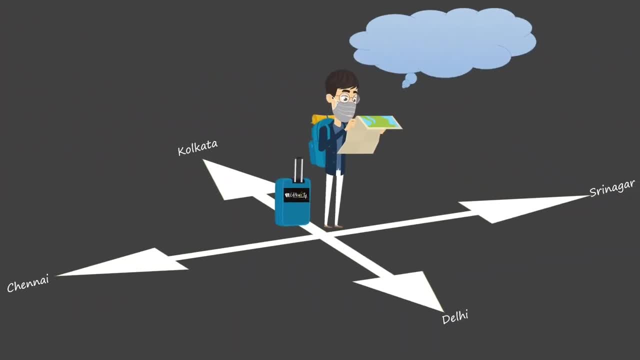 Let's imagine that there is a salesman who wishes to visit various cities in order to build his customers and sell his products. He has to visit all the cities exactly once and return back to his city in such a way that he spends the minimum amount of money possible. What is the best route he should take to minimise his costs? 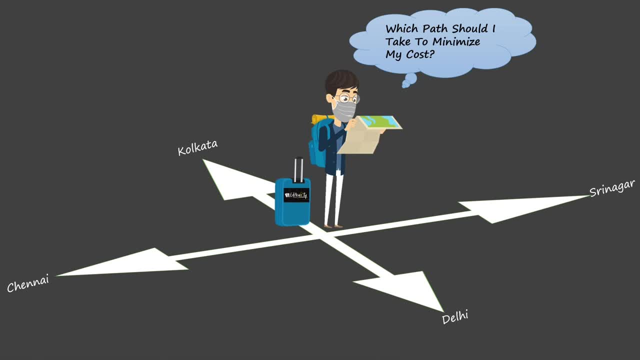 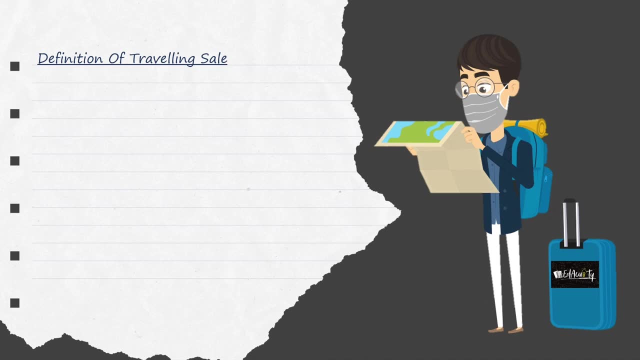 So there can be various possibilities to find the best path, And this is exactly where maths comes into play. Let us now have a look into the definition of the travelling salesman problem. It states that, given a list of cities and the distances between each pair of cities, 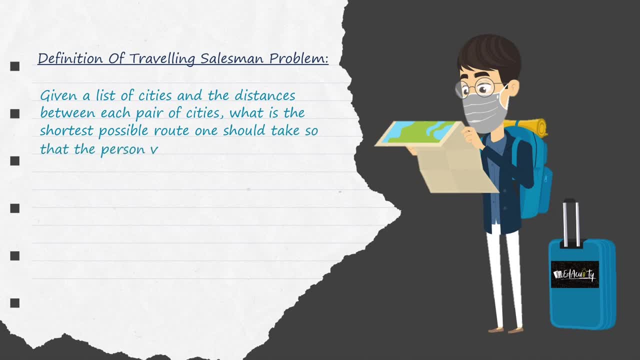 what is the shortest possible route one should take so that the person visits each city exactly once and returns back to the original city, by minimising various constraints, ie the time taken, the travelling cost and the distance travelled. The total number of possible routes for travelling between n cities where there is an edge between: 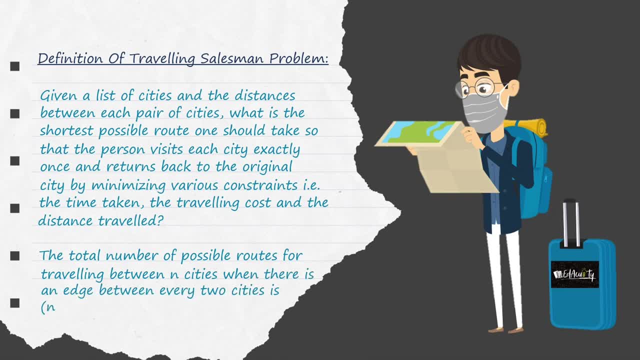 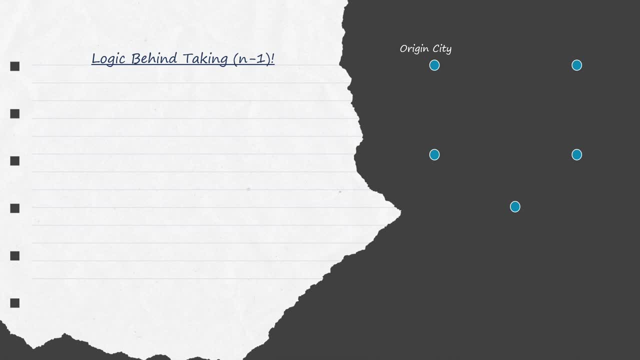 every two cities is n-1 factorial. Want to know the logic behind taking n-1 factorial? Well, we know that there are n cities in total and the salesman has to start his journey from the Origin City and end his journey at the same city itself. 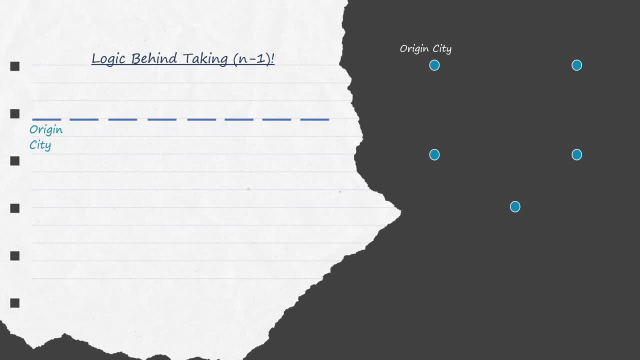 That means the Origin City is both the initial and the final point of the journey. For starting the trip, the person has only ONE option, ie start from the Origin. We know that the person is required to visit every city only once and there is a path between every city, so to traverse to the second city. 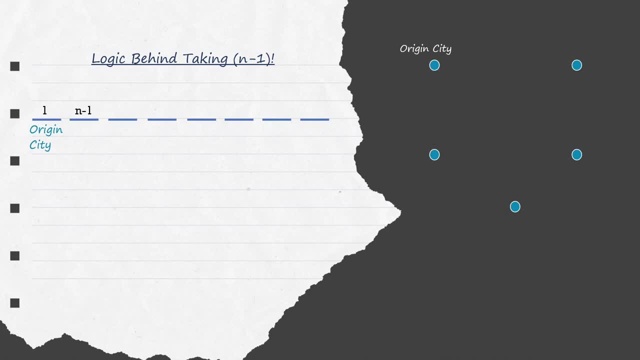 left with n-1 options, As we can see that he has covered two cities, so to traverse to the third city, he has n-2 cities to choose from. Similarly, the number of cities goes on decreasing by one as the person traverses. By the end he is left with only one city. 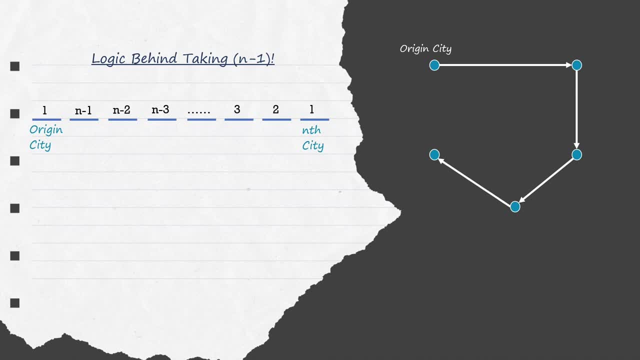 to traverse to, that is, the nth city, Since no city is left to be traversed, so the person goes back to the origin. Thus the total number of possible roots will be calculated by multiplying 1, n-1, n-2 till 1, and thus we get n-1 factorial roots. 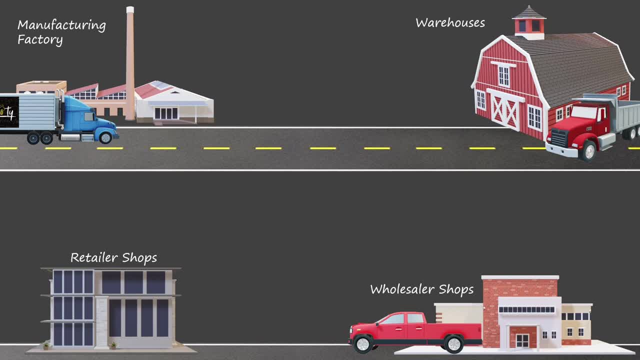 Now coming back to our question: how does this work in case of a delivery system of the manufacturing company? There are five basic stages in which the goods are being delivered. Firstly, the products made in the factory are supposed to be transported to the warehouses of the company From the 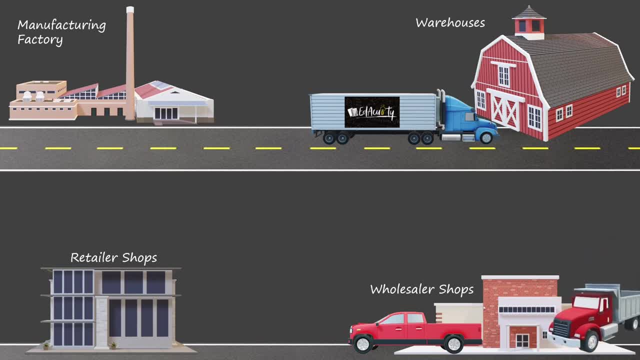 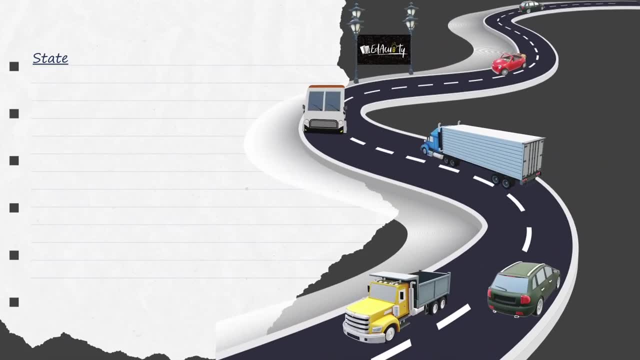 warehouses, they are to be transported to the wholesalers, from the wholesalers to the retail shopkeepers and then, finally, to the customers. Let us understand by considering the following problem, which can be stated as a manufacturing company situated in Surat has to send its goods to the warehouses situated in three different 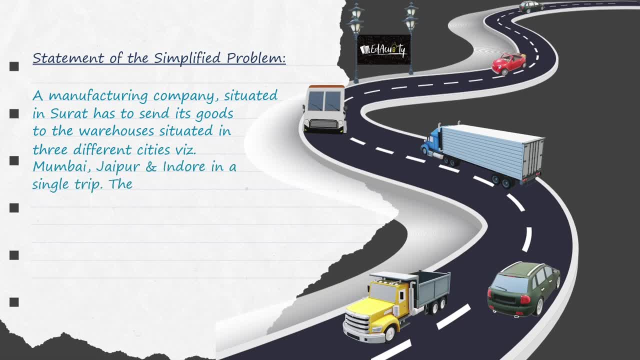 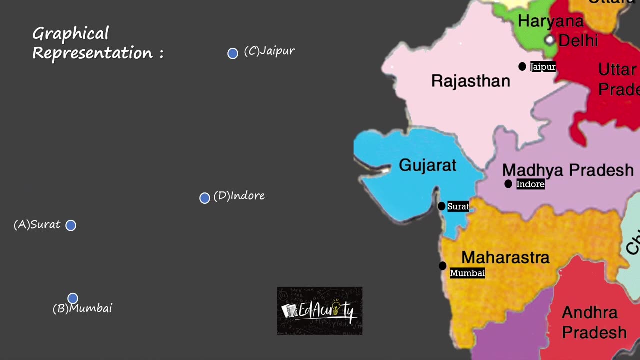 cities with Mumbai, Jaipur and Indore in a single trip. The company aims to minimize the total transportation cost. What route the company should opt to have the minimum transportation cost? On the right hand side you can see the positions of the four cities: Surat, Mumbai, Jaipur and. 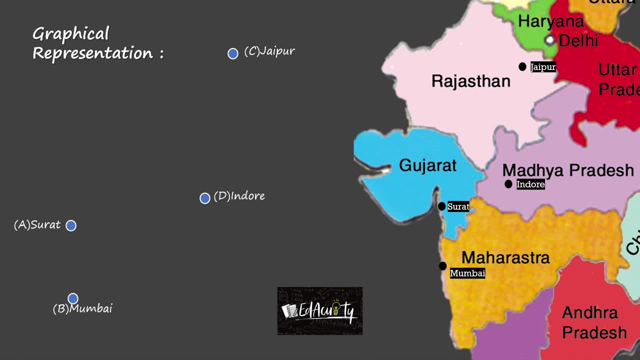 Indore, corresponding to their locations on the map of India. Besides, this is the graphical representation of these cities, which are being shown as the vertices of the graph denoted as A, B, C and D respectively, and the edges between them represent that there is a route. 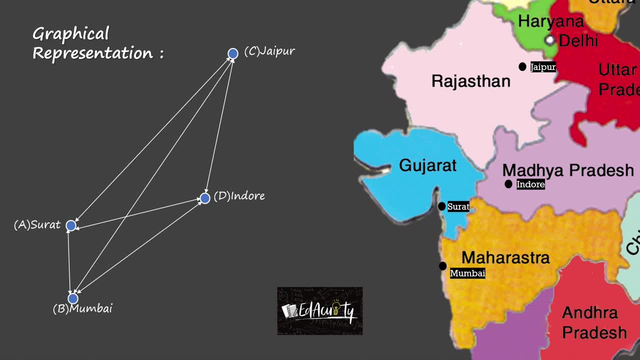 between the respective cities. You will see that each city is connected to every other city by an edge. In graph theory, where there is an edge between every pair of vertices, it is called a complete graph. In fact, any map can be converted into a graph with no more than four colors in it. 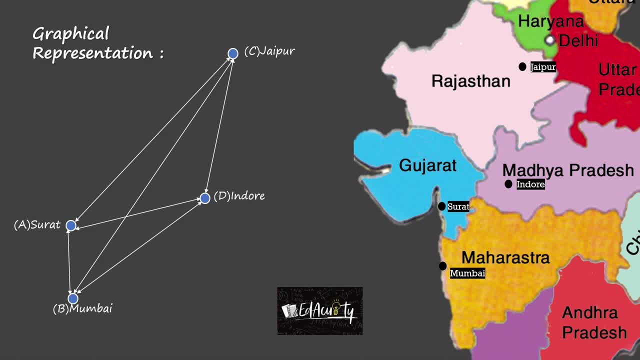 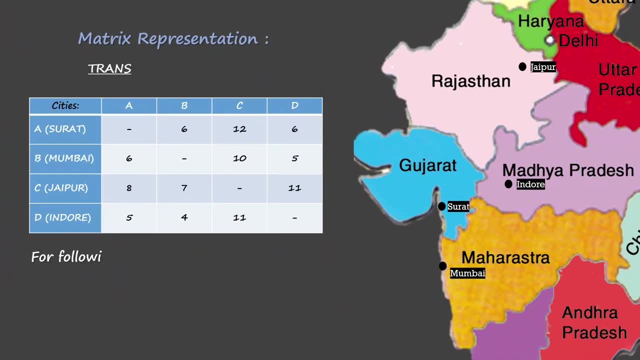 such that no two adjacent regions have the same color. Interestingly, this is known as the famous four color theorem. This is the matrix representation corresponding to our problem. The costs incurred for travelling between the two cities are given, where one unit is considered to be equal to thousand. 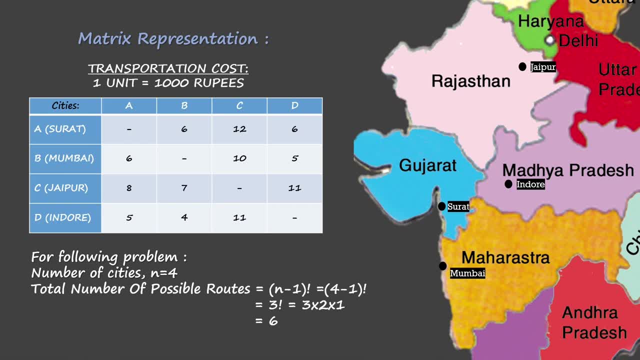 rupees. You can see the elements of the matrix, which are the transportation costs associated with every edge between the two cities. For example, the transportation cost from city A, that is, Surat, to city B, that is, Mumbai, is 6 units or 6000 rupees. Similarly, from Surat to city. 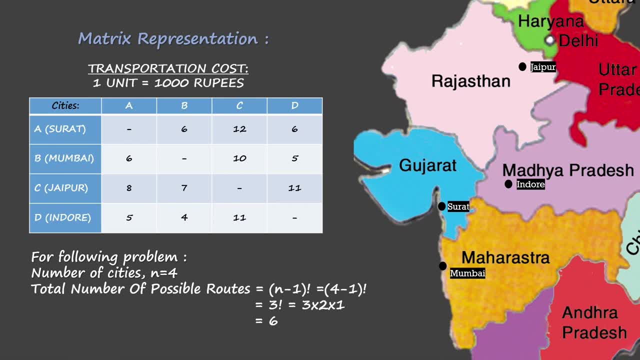 C, that is, Jaipur, is 12000 rupees, and from Surat to the city D, that is, Indore, is 6000 rupees, And the same goes for every other city. You must have understood why the transportation cost from a city to itself is not taken as 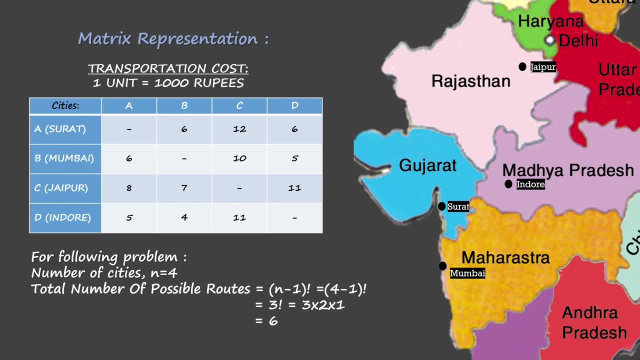 we are concerned about transportation from one city to another and not in the same city itself. We will be discussing in detail about its mathematical approach in our upcoming videos. Now we have to see how many possible routes can be there, As we have seen in the graphical. 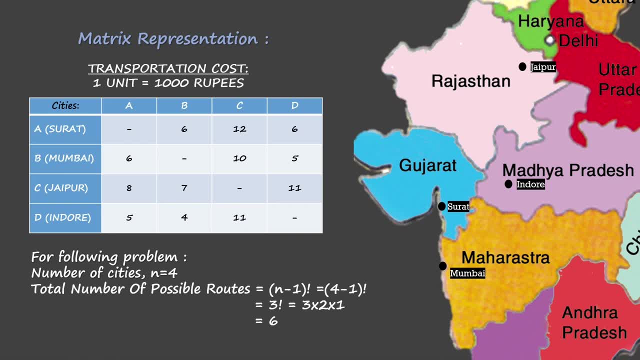 representation that there is a path between every two cities, We have to see how many possible routes can be there, As we have seen in the graphical representation that there is a path between every two cities, Since there are four cities, so the total number of routes possible will be 4-1!. which. 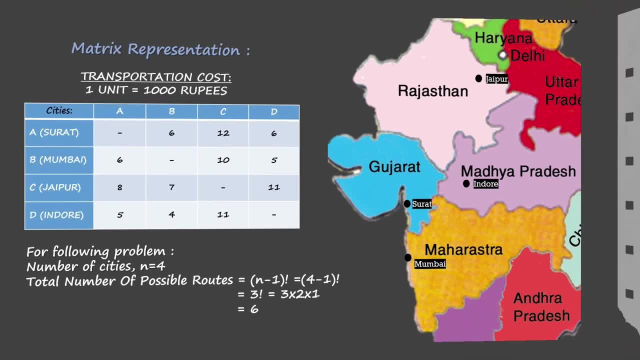 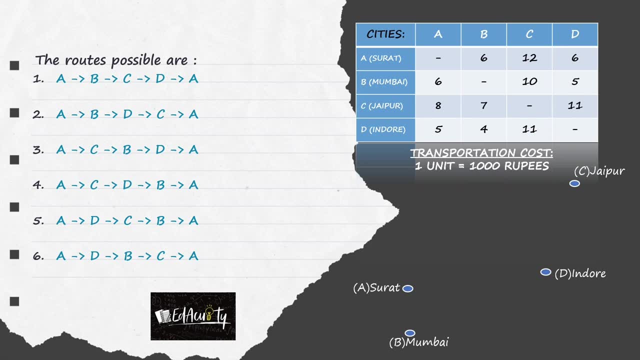 is 3!, which is equal to 6.. Now let us find the transportation costs associated with each route. Here you can see all the six possible combinations of the routes. The very first route is A to B, B to C, C to D. 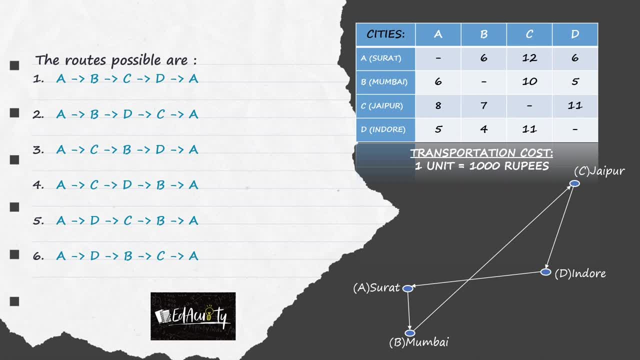 D to A, That is the manufacturing factory. The manufacturing factory will first transport its goods from Surat to Mumbai, then from Mumbai to Jaipur, Jaipur to Indore and from Indore it comes back to Surat. Now the costs corresponding to each path, which are being given in the table, will be added. 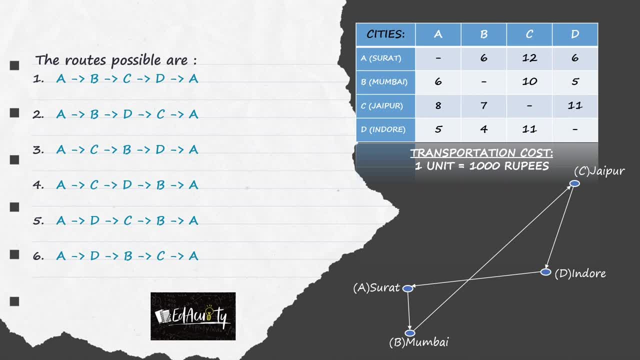 up together and in this way will get the total costs incurred in a route. So the cost corresponding to the first route is Rs 32000.. You can pause the video here and carefully check the other possible routes as well. Here in which there is a fifth route. 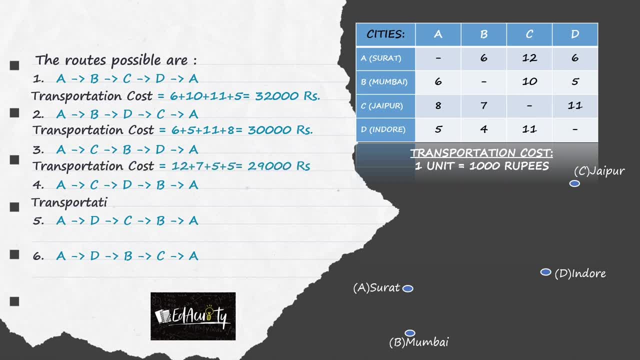 You can agree that the minimum cus수 cost for each route will be Rs 6万, Size 151.. Here, for example, theść corresponding to either route is Rs 4, Ku drift from UR 5 to UR6.. The costs corresponding to the second route is Rs 30,000, to the third route Rs 29,000.. to the fourth route it's Rs 33,000, to the fifth route Rs 30,000 and to the sixth route it's Rs 28,000.. Now see that the minimum cus수 of CCP politics, which is associated with